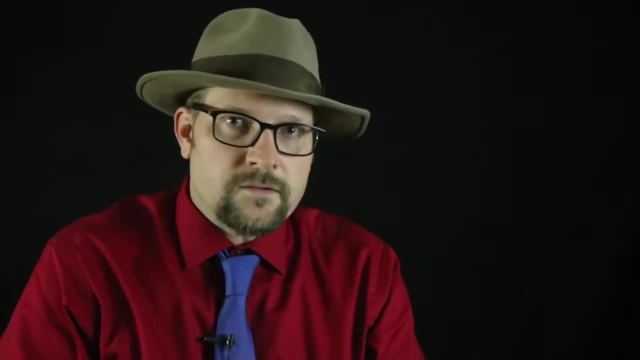 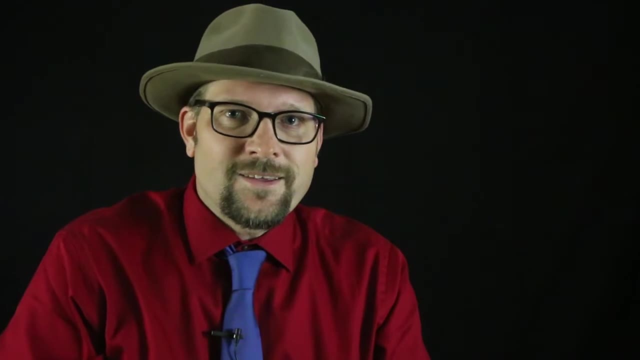 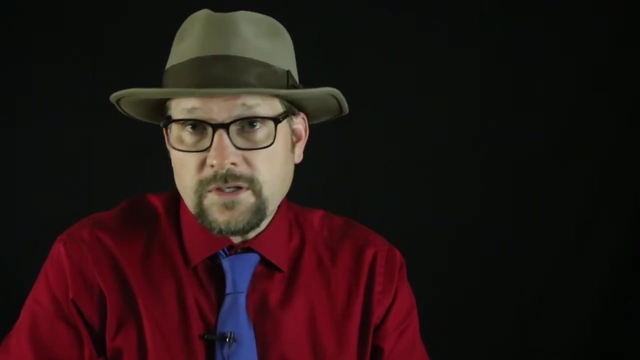 Welcome to Utah State University's Vertebrate Paleontology course. My name is Benjamin Berger and throughout this semester I'll be taking you on a journey to learn more about the fossil record of animals with backbones, from the fossil record of fish through early amphibians. 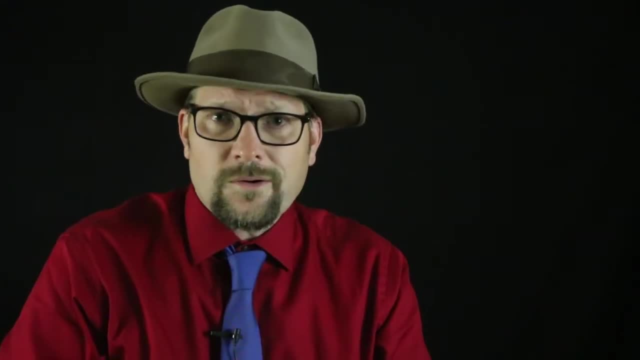 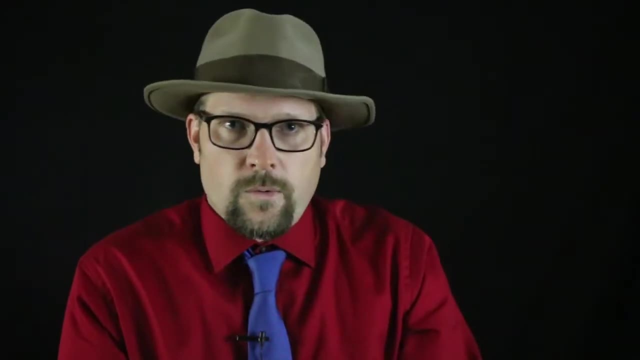 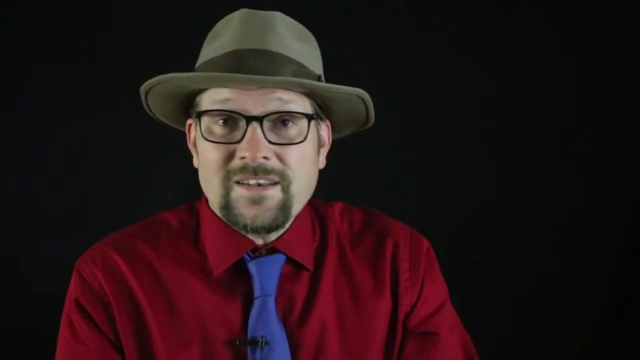 primitive reptiles, dinosaurs, pterosaurs, birds and mammals, including the fossil record of humans. This is a survey course, since each of these groups could be their own course to themselves. In fact, I teach a Natural History of dinosaurs course at USU. 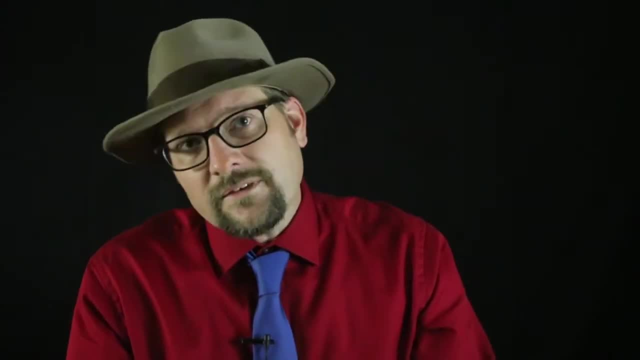 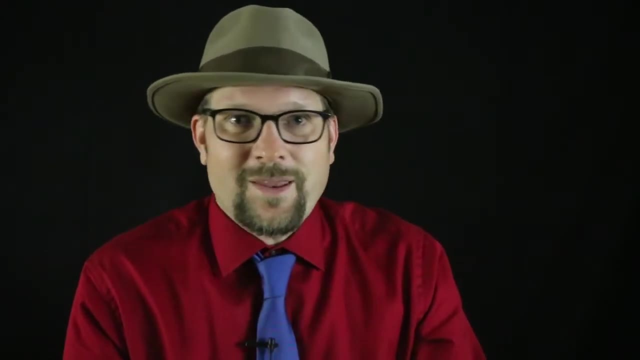 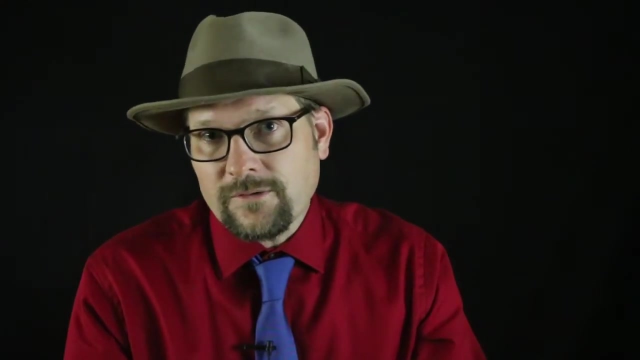 for which you find videos on YouTube. So with this class, I really spent more time on fossil fish, amphibians, reptiles, birds and mammals that are more often less well known, though, than dinosaurs, Although I have expanded the lectures on dinosaurs somewhat so we can cover that group in this. 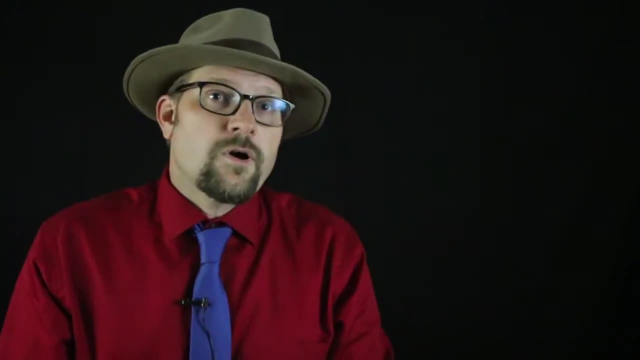 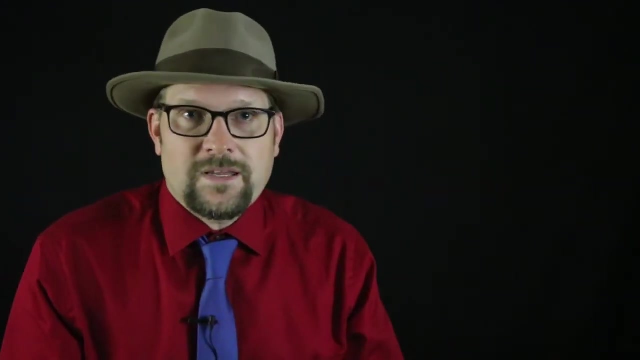 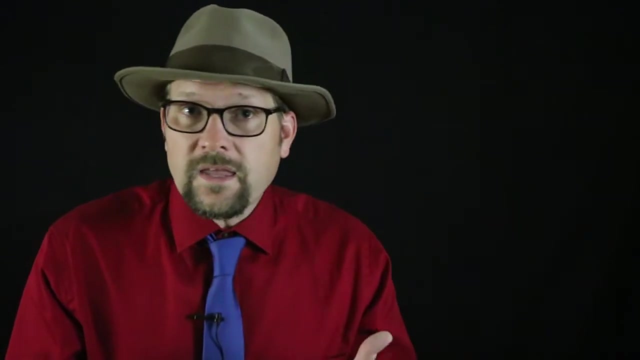 class in modest detail. Overall, we are going to be moving very quickly in this class and I have picked the major concepts within each group, really focusing on the controversies, the terminology and the current thinking in the evolution of vertebrate animals, with the hope that, if you want to, 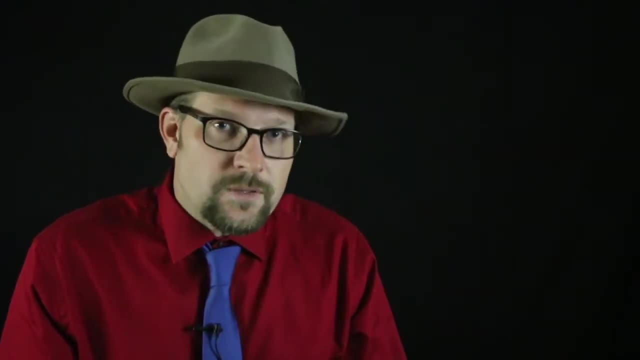 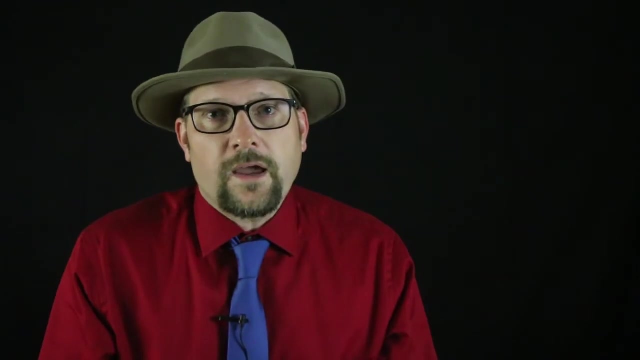 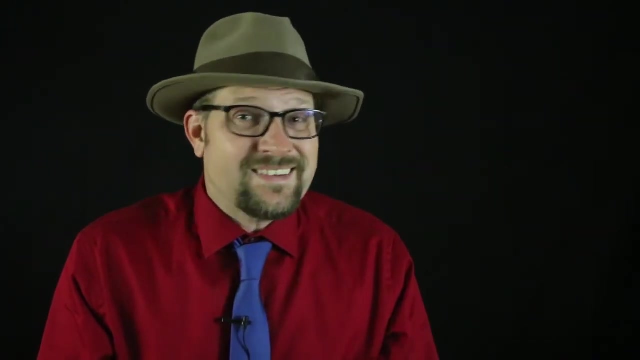 learn more, you will be well prepared to read more deeply into the primary literature I have been teaching here at USU for five years now. I have collected vertebrate fossils from half a dozen natural history museums here in the United States since 1995.. 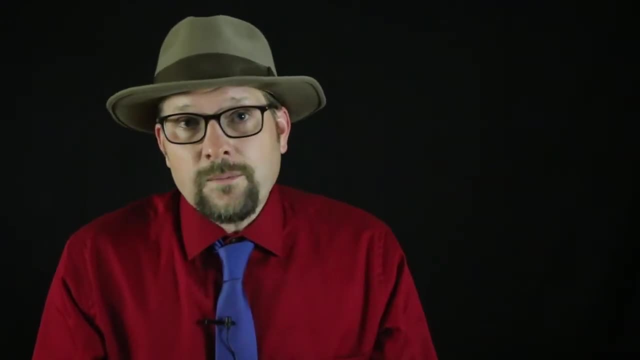 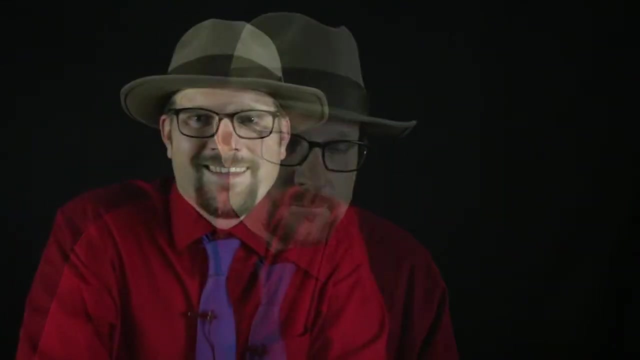 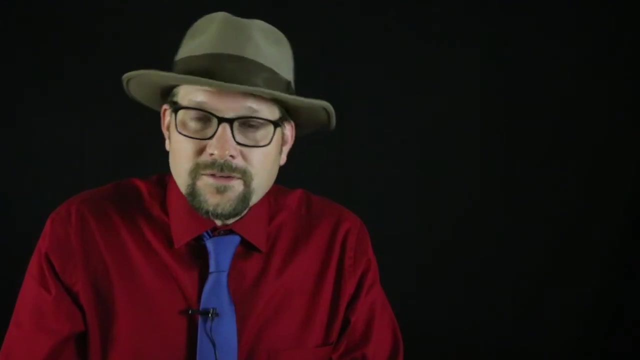 I have got degrees in geology and anatomy and I have taken many courses on vertebrate paleontology and vertebrate comparative anatomy. Okay, My expertise is on fossil mammals, so we will explore and expand on those groups in this class. I have also been working on the fossil record of mammals here in Utah, as well as in Wyoming.